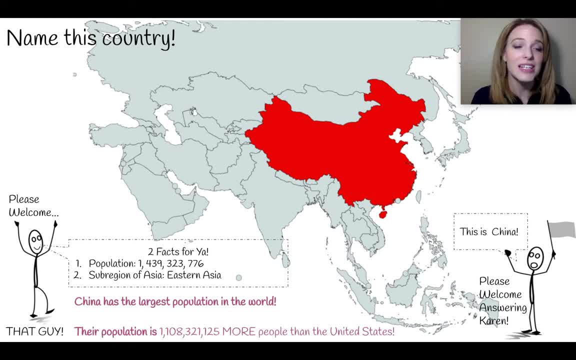 on. So please welcome that guy. He's going to be the one Giving us interesting facts and medical to do the math. today, in 2020, says China has the largest population in the world, and this population is 1 billion 108 million 321 thousand 125 more people. 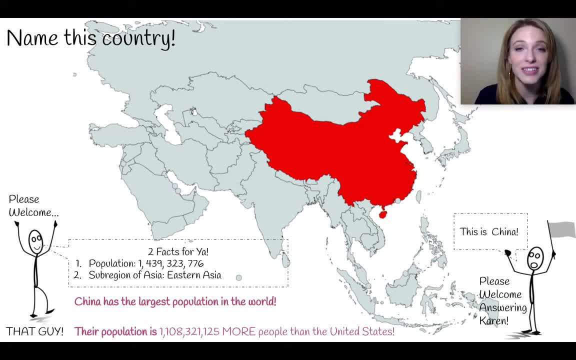 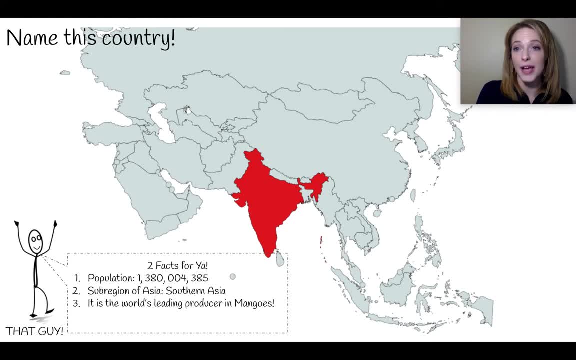 than in the United States. that is absolutely astounding. can you name this country? so this country is known for trade, as well as a couple other really large things like Hinduism, but it's also known for mangoes. okay, so correct, you got it. this is most definitely India. this is hey, Karen, go along. so when we 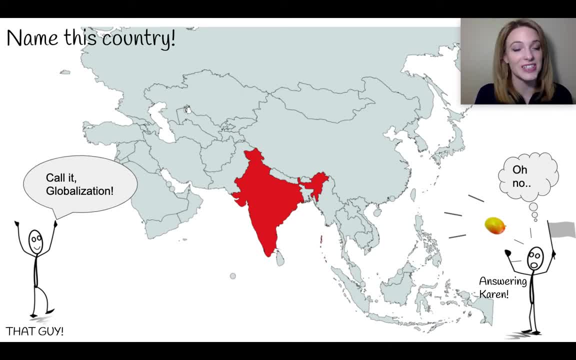 talk about trade, we do know that it is globalization on a massive scale, and so that does play a leading role in connecting these countries with one another. so trade plays a significant role on global economy. India is the ninth largest trading partner. now I'm sure you know this one as well. we've talked about it in class. we talked about how it was. 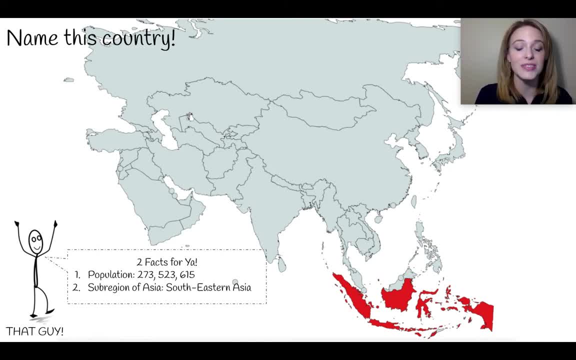 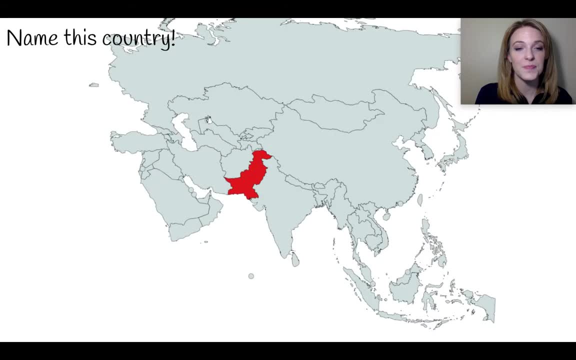 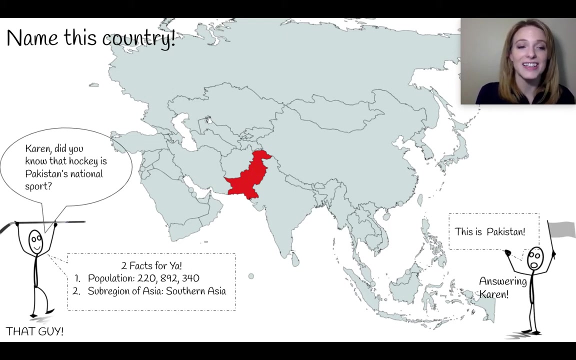 an archipelago had a lot of volcanoes. do you know it? good, it's Indonesia. this one, this one's pretty cool too. this one is definitely one you need to know. it's Pakistan, but one interesting fact you probably didn't know is that it is known for hockey. it's the national sport there. 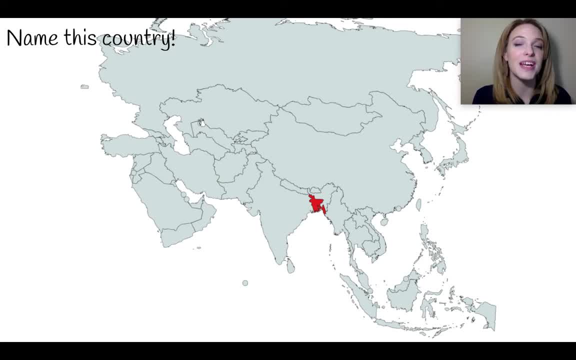 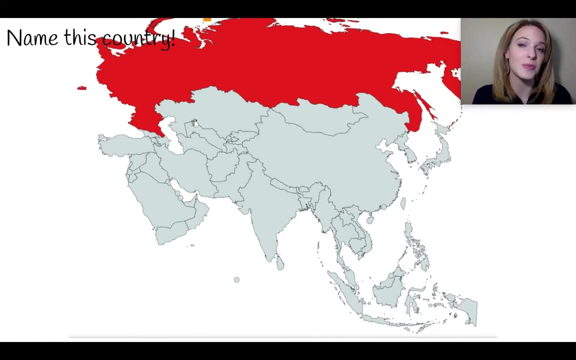 okay, can you name this country? it's quite small, but it has one of the world's largest populations. good job, that's Bangladesh. all right, what about this one? I bet you thought this one would be earlier, but it's actually not. I bet me it's a lot of these zines, just because each one has its own similar. 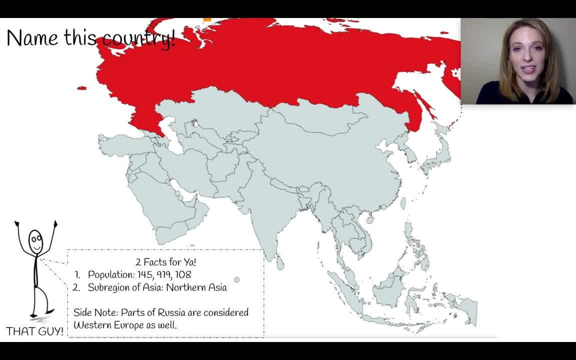 yddities, and they have the same name on the damaged area of the map. so if you want to know about other groups of countries, you can check out these now. today I'm going to be doing a pretty fun. 내가 intro, okay, so this is where. 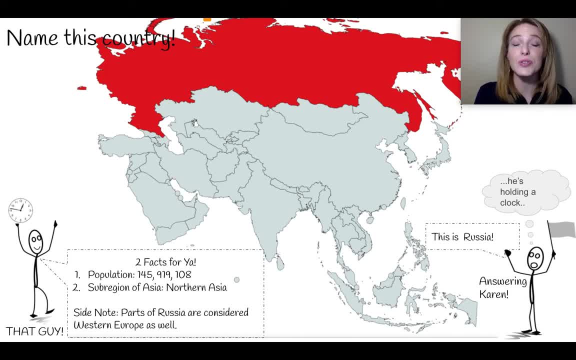 we find Western culture and they can be shown in foreign-게요 cultures. so this is a good punt of key romance. before we start, we have precon checks, which is we can actually see Russian culture from all over the world. but yeah, this is critical. gusto talk a lot about both such history and how people lived up to Russia today. 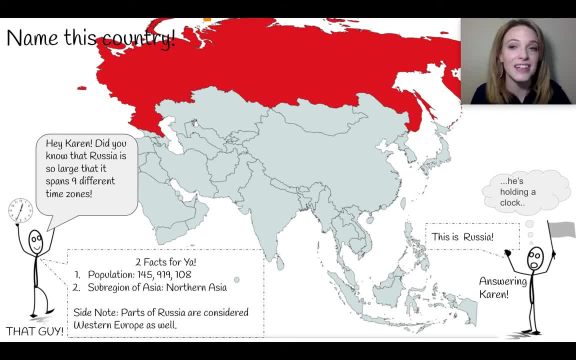 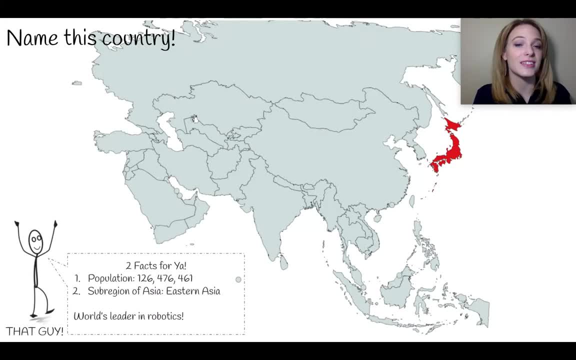 call a family member who also lives in Russia and be at nine hours apart. It's crazy. So can you name this country? You can? The world's largest in robotics. Good job, You got it. Japan, How about this one? It's next to Indonesia, Also has a lot of 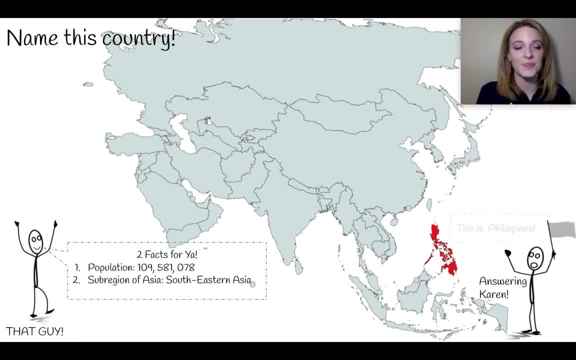 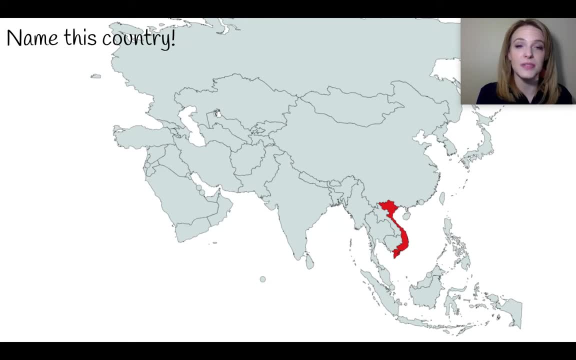 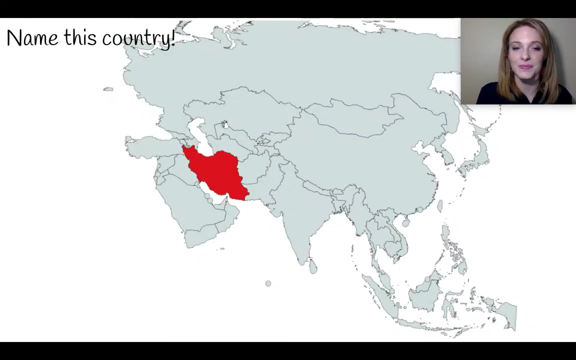 islands with it. You got it: The Philippines And this one. many of your relatives, maybe, a generation ago, could have played a role in this war. Good job, It's Vietnam. What about this one? Okay, We still have a really high population at this point in time, So we still have a lot of. 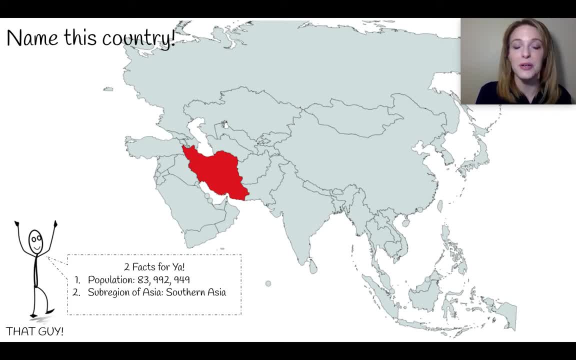 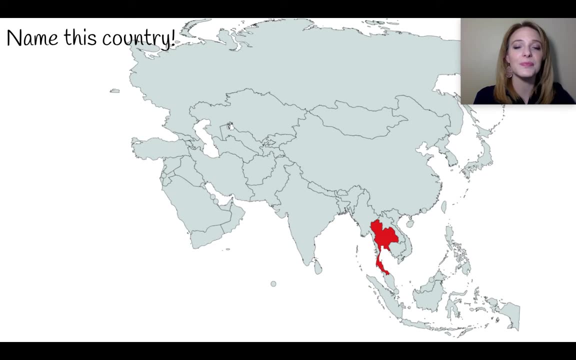 people. We still have 83 million. Okay, We're going down progressively, but these are countries with a lot of people. Did you get it? Iran? Good, Okay, Can you name this country? It's a very unique shape, doesn't it? Okay, It is known for having the world's smallest mammal, And I bet. 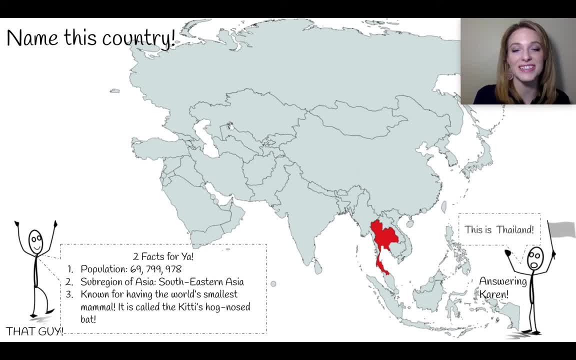 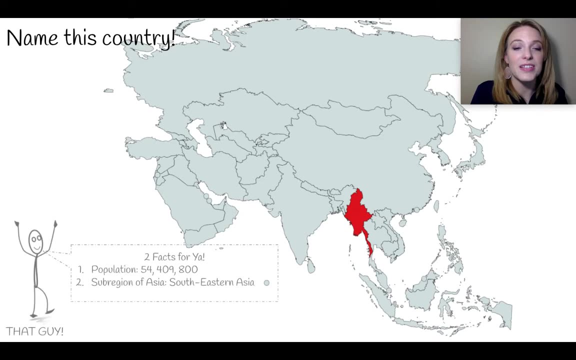 I don't know if you've seen it. Look at this. Look how small it is. It's in Thailand Now. I know, with everything that's happened with the pandemic, there's probably some people who are skittish or fat, but I find this little mammal very cute. So this: 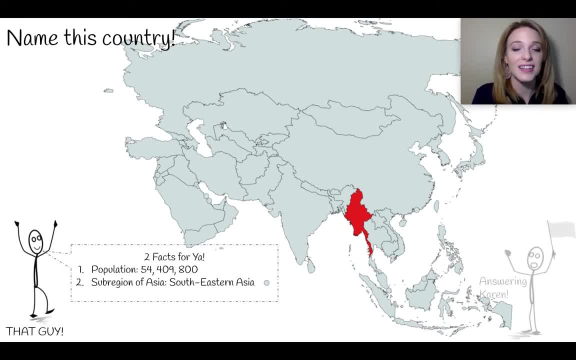 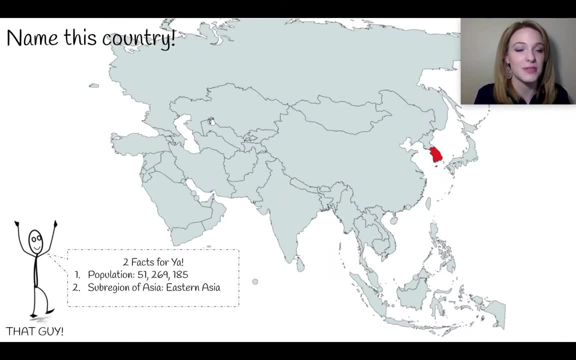 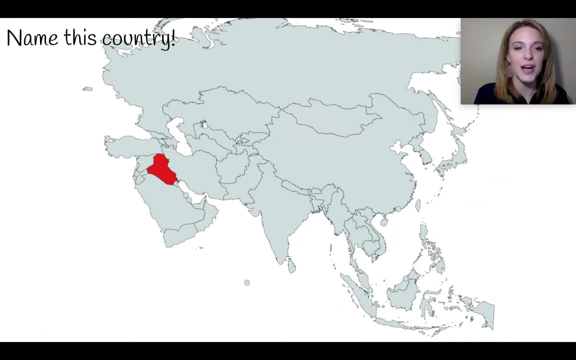 country, can you guess it? Okay, Good, Myanmar. I bet you know this one. We talked about this one quite a bit. Good job South Korea. What about this one? Can you figure it out? Good job Iraq, Also known as the cradle of civilization. 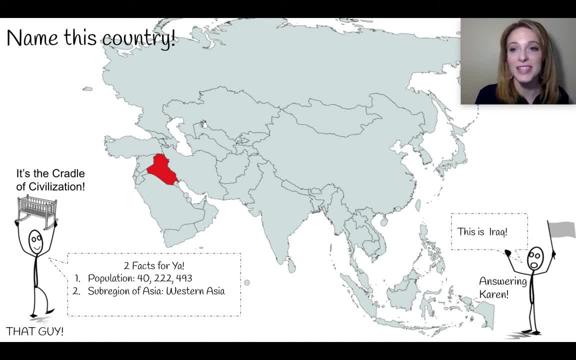 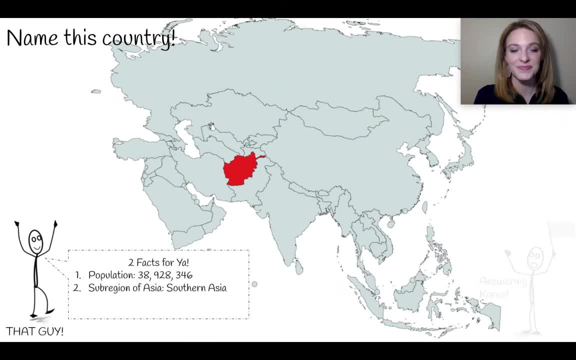 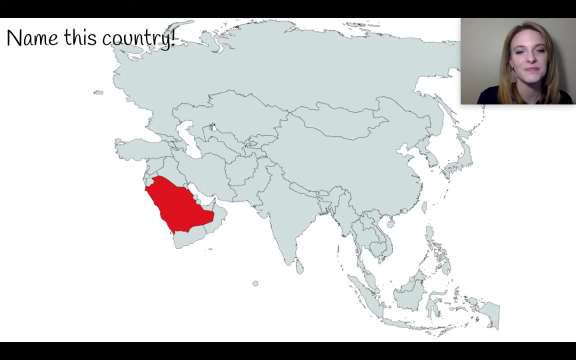 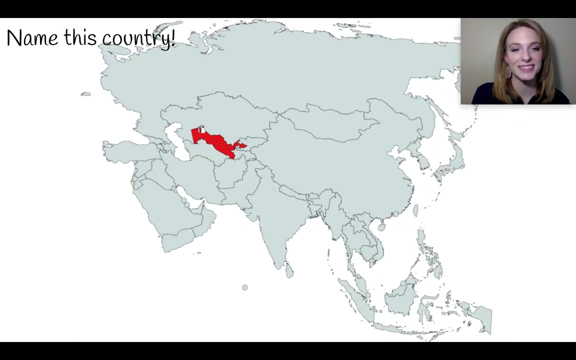 Very important. So you have the tigers and the Ubranis. Can you name this country, Afghanistan? Good job. What about this one? It's quite large, Also known for its oil, Do you know it? Good job, Saudi Arabia. And this one, What's Karen going to say? Good job, Uzbekistan. 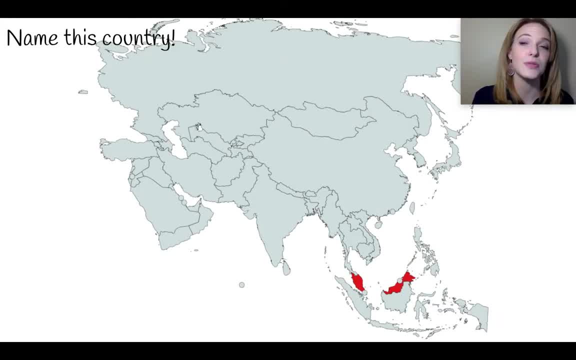 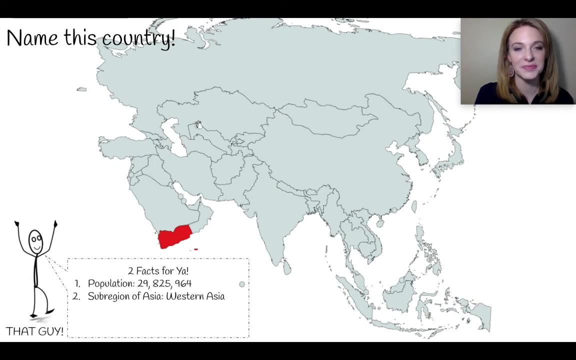 Now this one. if you'll notice, it's in two almost drastically different locations. It has massive body of water in between. So Malaysia for sure. What's this one? Yemen? I find this funny and you'll notice it in a second, but Yemen is right next to another one, that's. 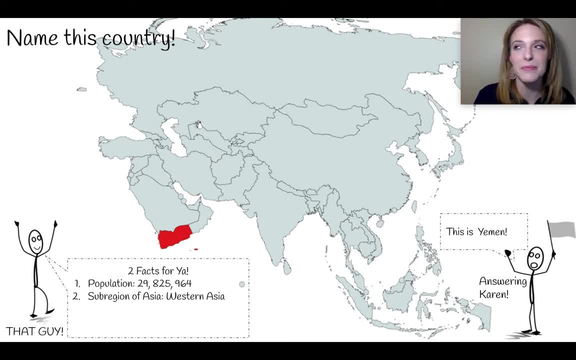 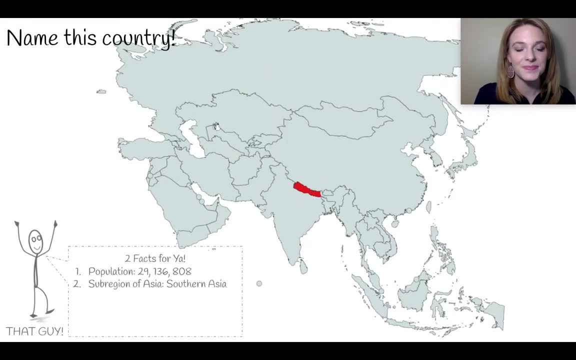 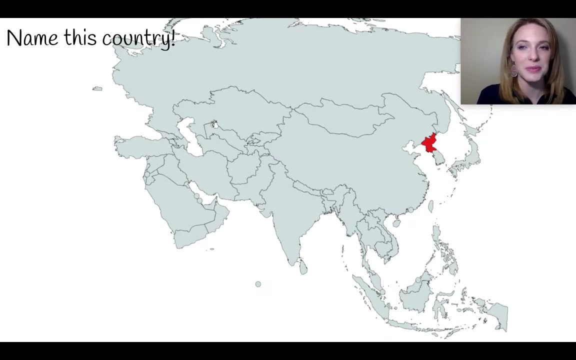 very similar to it, So it almost makes me feel like I'm speaking Jamaican, And it's just funny. I wish I could not, but I love their accent. Okay, Do you know this one? It's right above India, Nepal, Good job. What about this one? I'm positive you should know this one. Now. we talked about 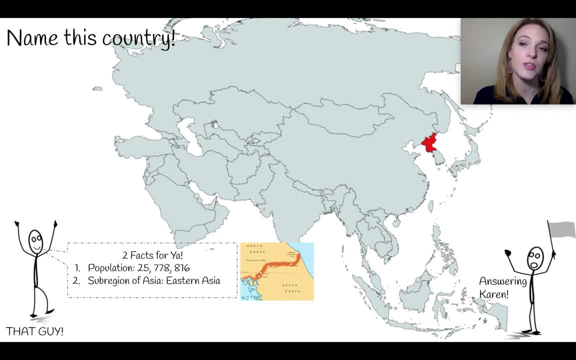 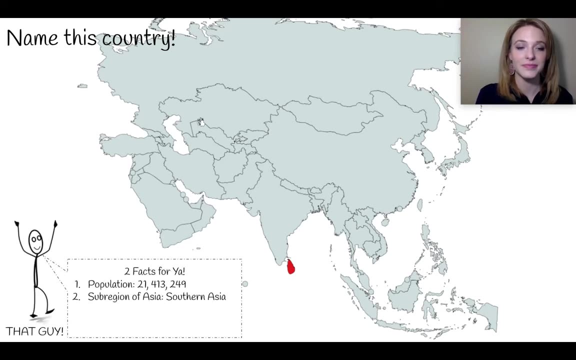 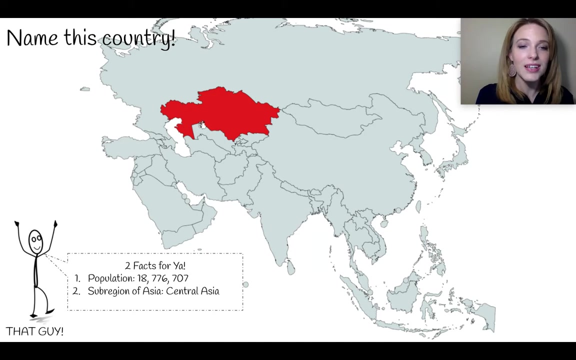 this one before. It's North Korea, Where they're trying to reduce the amount of warfare located there. Good, It's North Korea. What about this one Down below India? Good Sri Lanka. What about this one Right underneath Russia? This one's been hot the bay. Kazakhstan. Good job Kazakhstan. 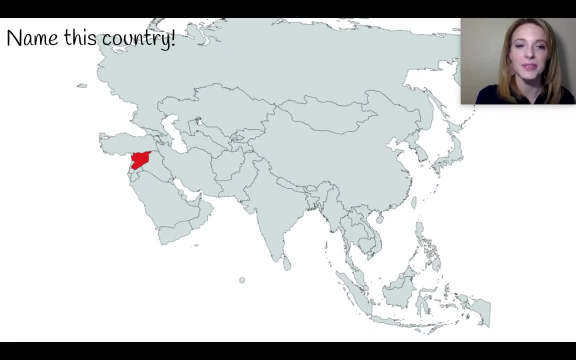 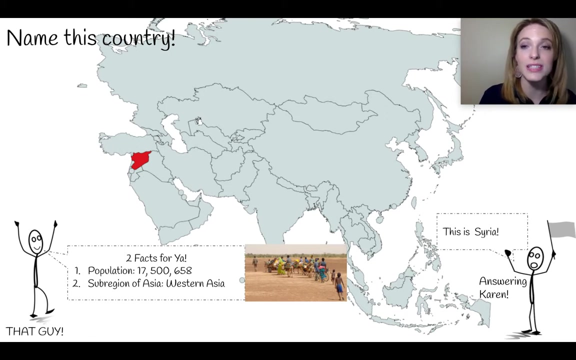 Good job. What about this one? It's definitely in the Western portion of Asia. Got it Syria, Oh man, oh man. Is that one important? We've talked about the Syrian refugee crisis and we talked about how desperate these individuals were to escape to an area which was 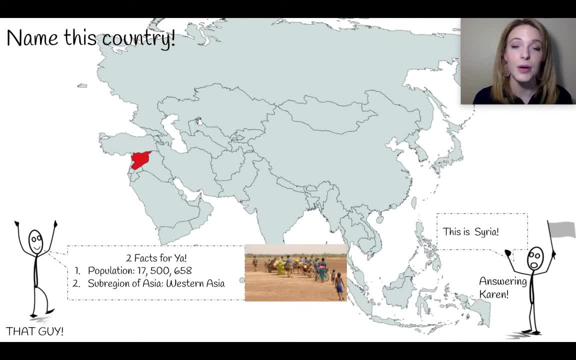 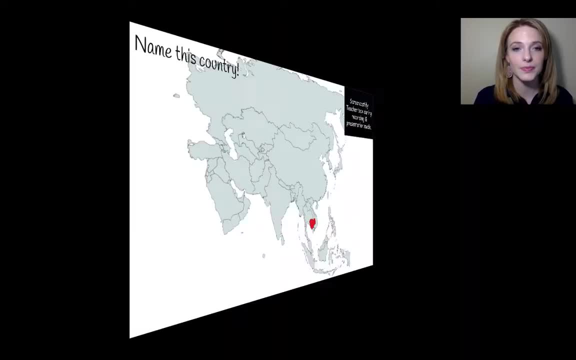 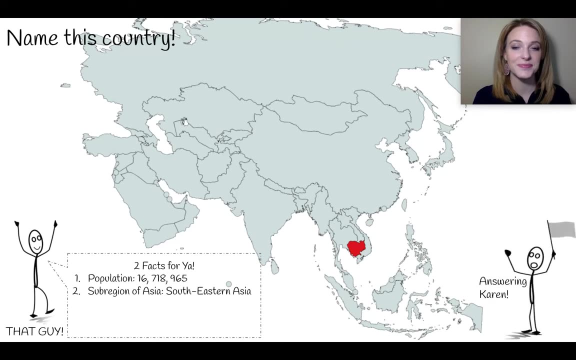 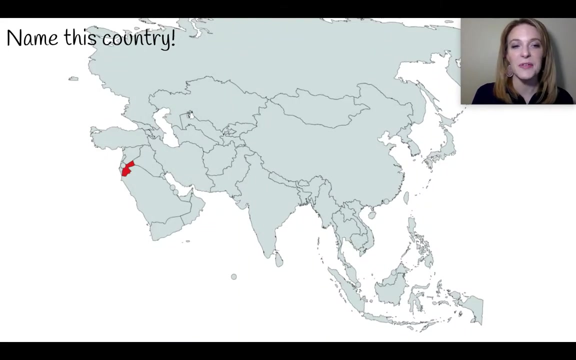 freer, but also how that definitely imposed some concerns within the countries that the refugees had to go through. It is definitely something that we should be praying about. What about this country? Do you know it? Cambodia, Did you get it? What about this tiny little one right here? 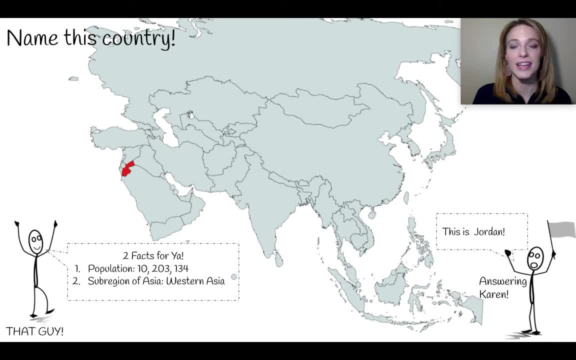 Okay, That's the Jordan. They actually get along better With Israel as opposed to many of the other nations and countries near them. Hey, Karen, did you know that? the lowest place in the world, having an elevation of 1,378 feet below? 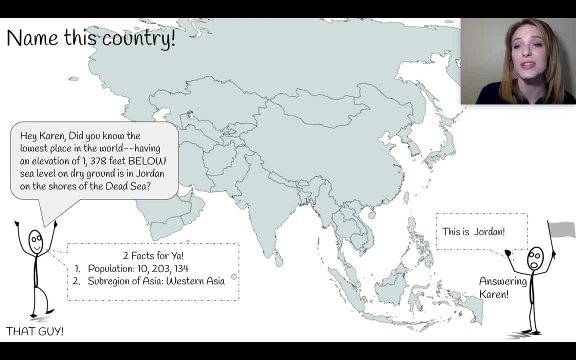 sea level on dry ground is in the Jordan on the shores of the Dead Sea. That is significantly lower. We live on the sea level right now here in the peninsula of Fort Lauderdale. Can you imagine going down lower, You know by a thousand plus feet, and still be on dry ground? the pressure would be different and it would be drastically different. 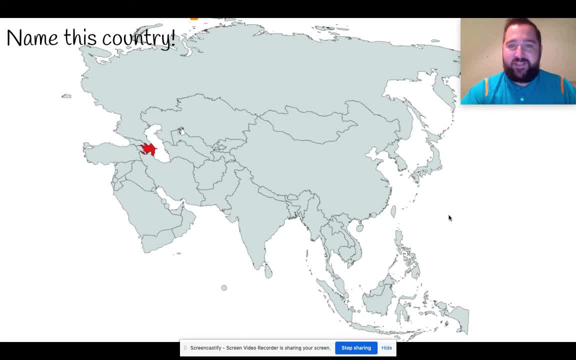 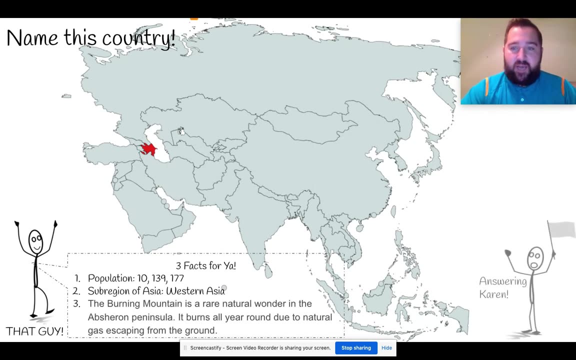 This is mr Boardy, and we're going to continue going through the countries, So let's jump right into it Here. you will see on your screen Marked: here is our new country. Let's give you some information. Here's some information, Wondering if you guys know the country. the country actually is. 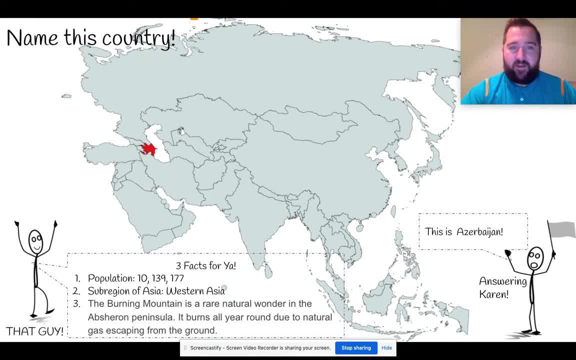 as you're, by John Azure, by John. Azerbaijan, here you see, has the population of 10 million hundred thirty nine thousand hundred seventy seven people. It's in the sub region of Asia, It's in Western Asia, And here, an interesting fact, that was pretty cool. Did you know here that the burning mountain 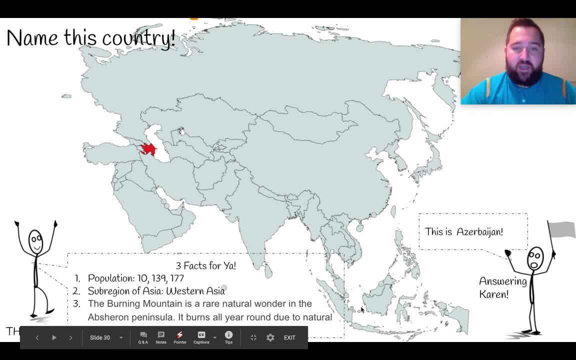 Actually is a area in Azerbaijan. The burning mountain is a rare natural wonder in the Abhijan Peninsula. It Burns all year round due to natural gas escaping from the ground. Here's a really cool image I thought I'd like to show you guys. 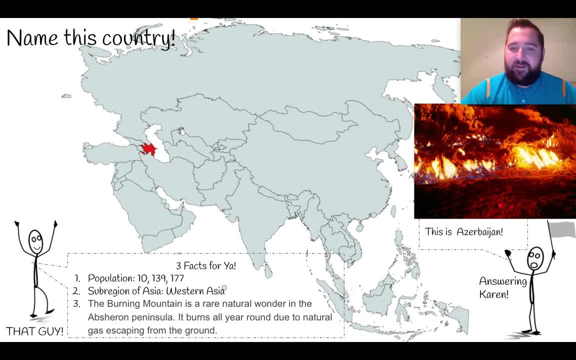 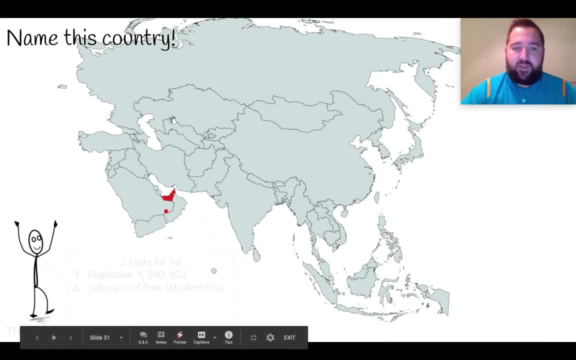 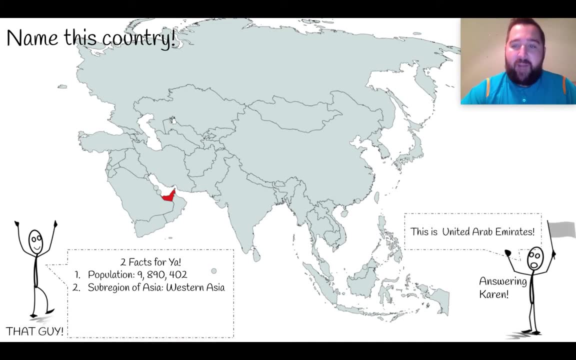 Let me click it. Here is the burning mountain. That was pretty cool. It burns all year round. Let's go to the next country, Next country label. here Here's some information. This country is United Arab Emirates. United Arab Arab Emirates, here Marked right here: population: nine million eight hundred ninety thousand four hundred two people. It's in Western Asia. Let's continue. 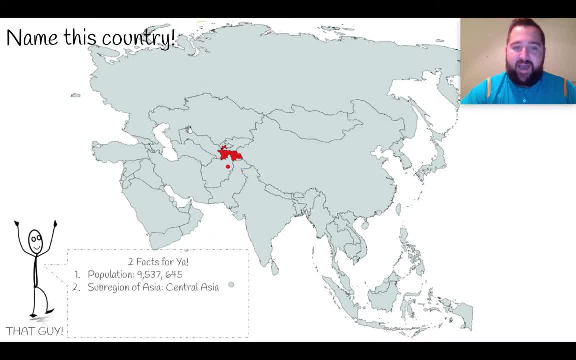 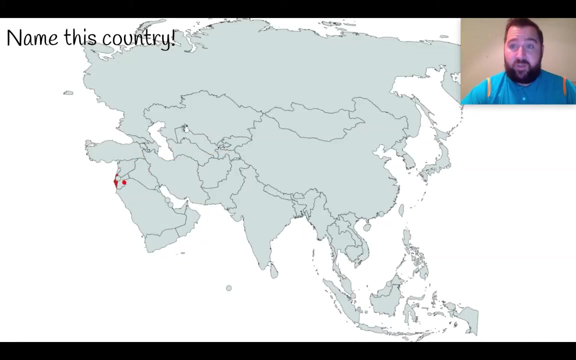 This country marked here, give you some facts. Do you guys know what country this is? This country is Kazakhstan, Kazakhstan. Kazakhstan, here, has a population of over nine million, five hundred thirty seven thousand. again in Central Asia and Next country over here on the corner. This should be familiar to you Definitely, as a Christian. this country is. 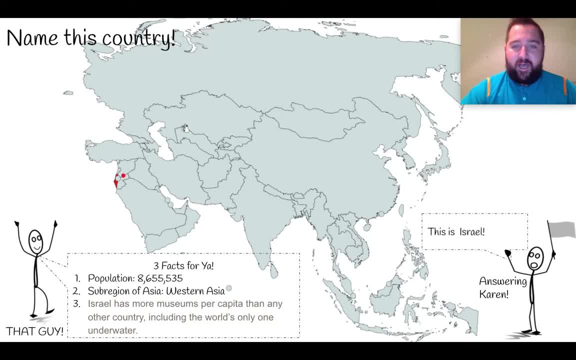 Israel, Israel here is Very important to us. definitely in the Old Testament We read about Israel all the time. Israel has more museums per capita than any other country in the world. They even have a museum underwater, So it's not saying has the most museums in the world. 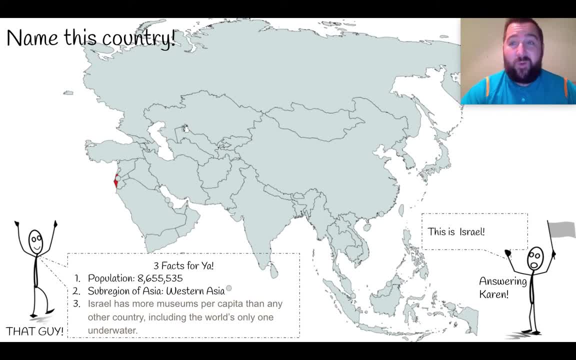 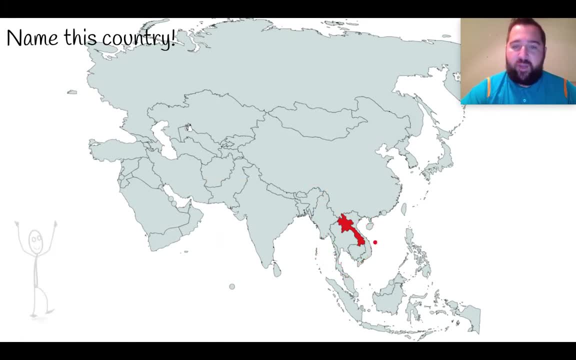 But for its size it has the most museums and even an underwater museum. but that was pretty cool. next to country, Here we have a new country marked for you. Does anybody know what that country is? that country is Laos. Laos- is this country right here in southeastern Asia? 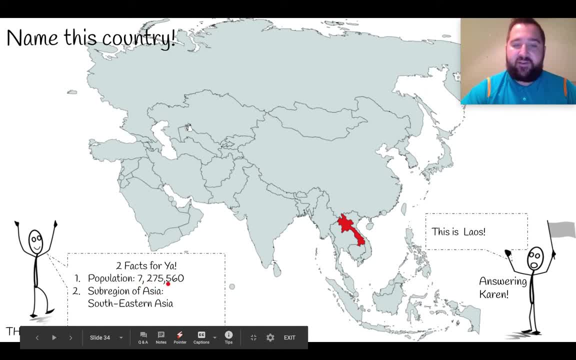 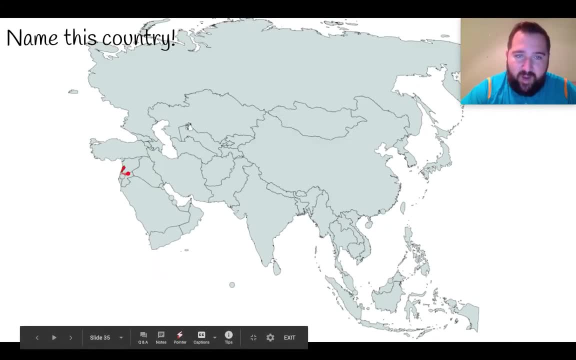 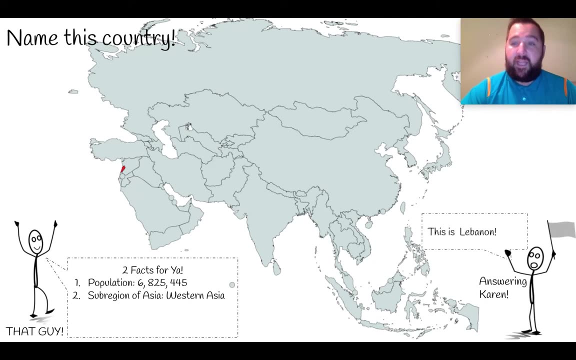 population of seven million two hundred seventy five thousand five hundred sixty. Laos- Laos, Next country, little guy you know, look close for it. little guy, right here, this country is Ready for anybody know it is Lebanon. Lebanon is the name of this country here. Awesome, let's keep going again. their population here: six million eight hundred twenty five thousand four hundred forty five people. 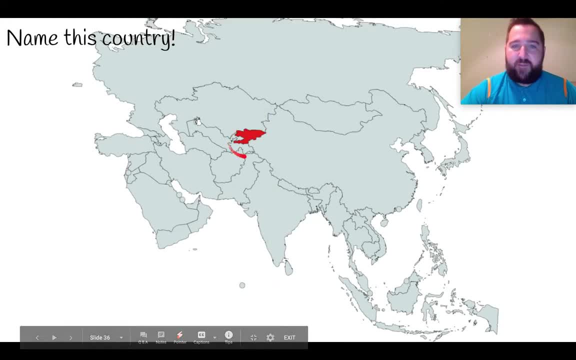 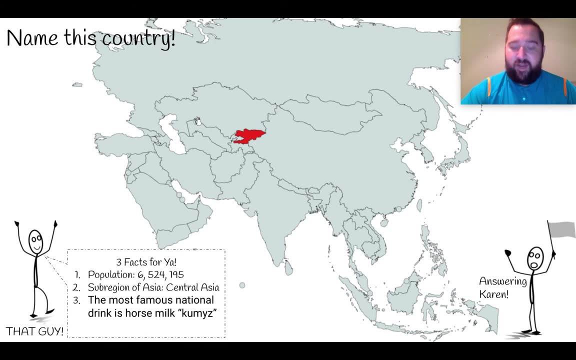 next country Up here on the top say: if I know what that is, That country is ready for it. Kyrgyzstan, Kyrgyzstan- I know it looks really weird pronunciation, but pronounced Kyrgyzstan Kyrgyzstan here- has population of over six million five hundred twenty four thousand hundred ninety five people. 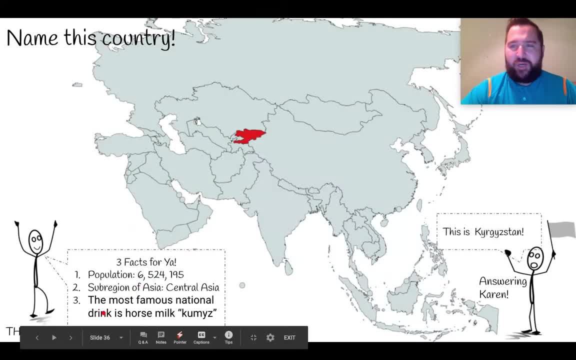 I found this really weird fact. I thought I would share it with you guys. the most famous national drink in all of Kyrgyzstan is horse milk, horse milk. I'm not going to be drinking horse milk any time soon. Don't know about you guys. 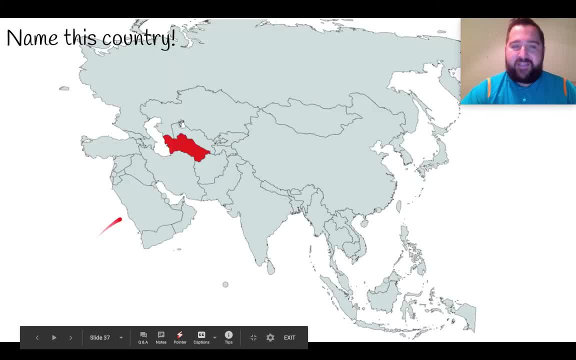 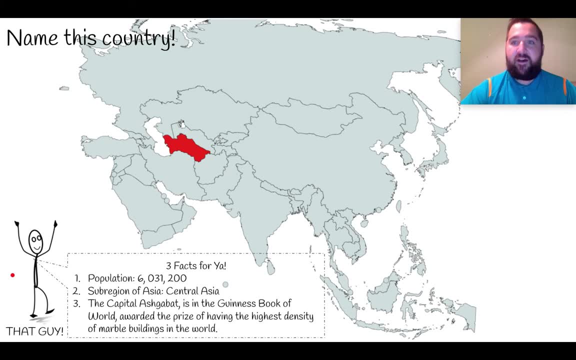 Next country. let's keep it going. Next country. you can see it marked here. See if anybody knows this one, This country is. anybody know This country is? It's pronounced Turkmen, Turkmenistan, so you know it says Turk. I've got it like T E R K: Turkmenistan, Turkmenistan. 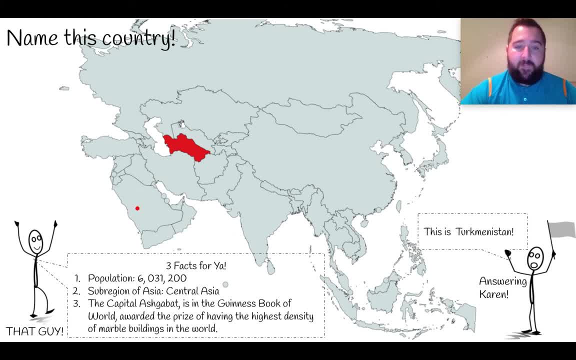 Here has population over six million people. It's in Central Asia. Look at this cool Fact, and that was a really cool fact: the capital of Turkmenistan is ashok robot. They're known in the Guinness World Guinness World Record. They're awarded a prize for having the highest density of the highest amount of marble buildings in the world. 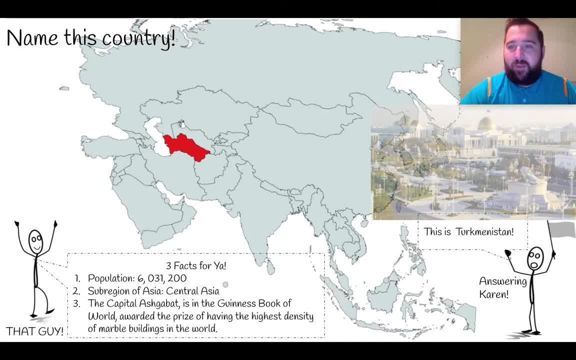 You guys can google this and kind of look at some of the buildings here. I want to show you an image of it. This is just one listed in Kyrgyzstan and kind of look at the buildings here if I want to show an image of it. this is just. 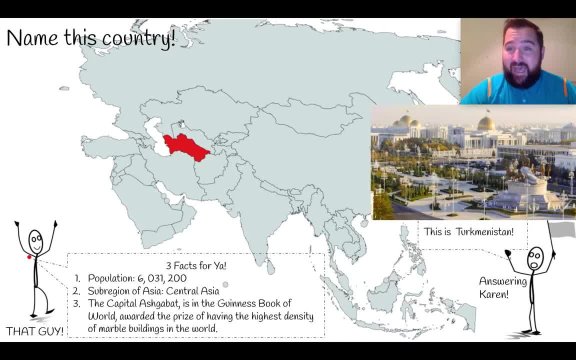 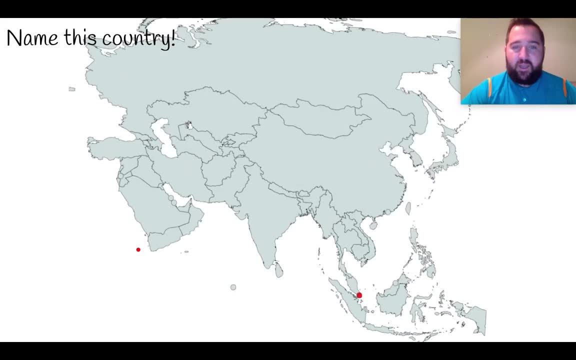 one image of all the marble buildings that they have from from lamp posts to fountains, to statues, to buildings- the largest amount of type of marble used in the entire world- thought that was kind of crazy fact. let's keep going. next country, you gotta look close for this one down here on the bottom, does anybody? 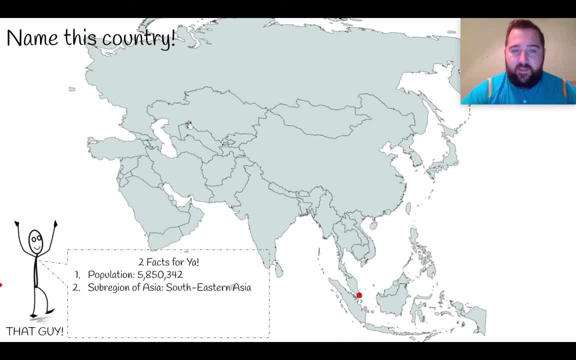 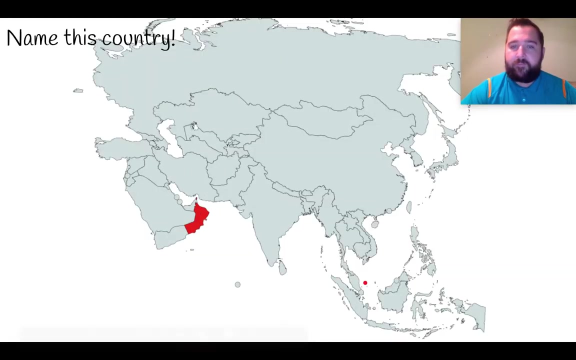 know what country that is. that country is Singapore. now, we've mentioned Singapore in some videos we talked about earlier last week. Singapore, even though they're small, look at their population: over 5 million, close to 6 million people there, and again, this is a southeastern Asia Singapore. next country, mark here: 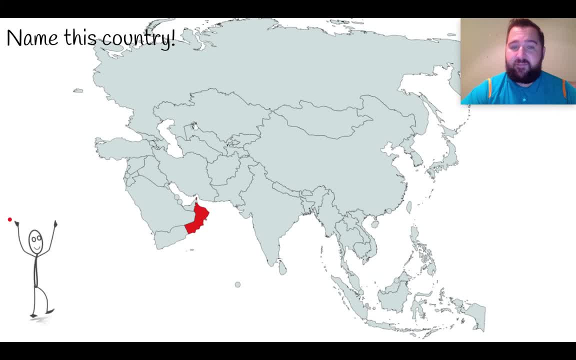 does anybody know what country that is? that country is Karen Oman. Oman, not to be confused with an eighth grader. Oman here is a very interesting and very awesome country. feel free to google. there's a lot of cool stuff about Oman, but for now we're just gonna keep going. 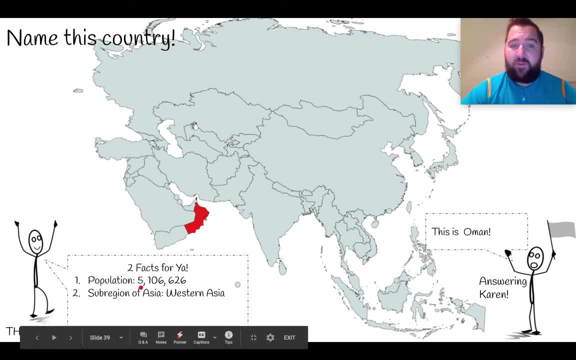 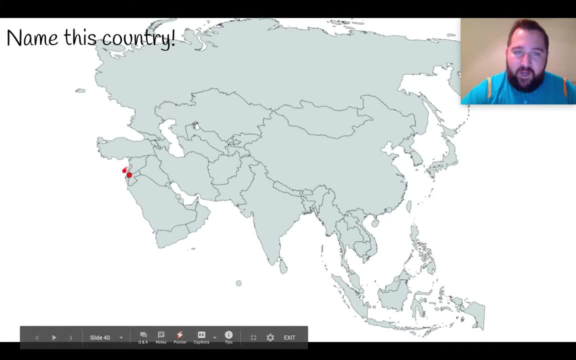 through the slideshow. they have a population of over 5 million people and it's also in Western Asia. let's keep going, you up here. a little tiny, little tiny dot near Israel. does anybody know what country that is? that country is Palestine. I know you've heard of the. 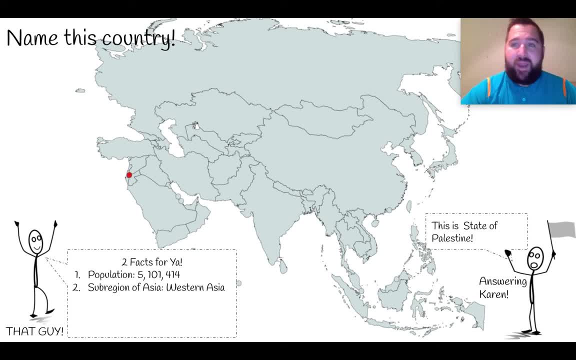 Palestinian conflict, or maybe I've mentioned that maybe in the news, or parents on the and Palestinian conflict. hopefully we'll get to that this unit, but here is in Palestine. their population is over 5 million 101,000, 414 people again in Western Asia, Palestine. 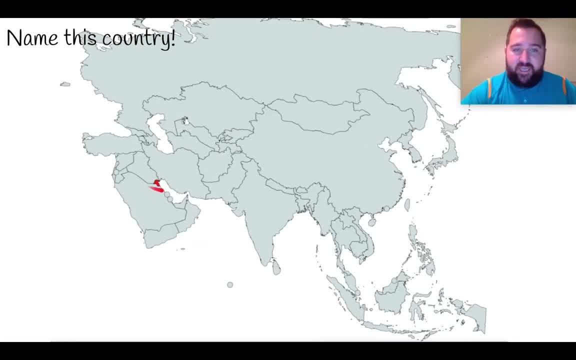 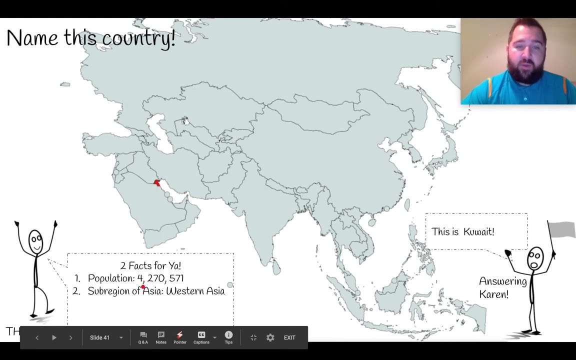 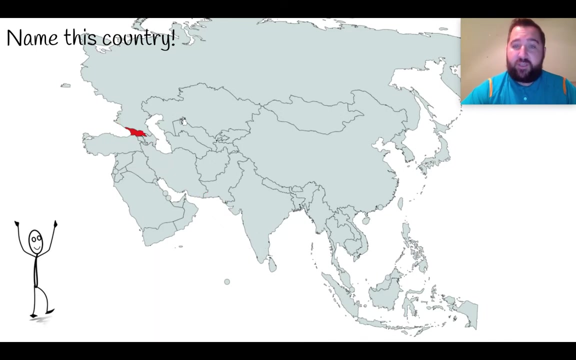 you got a little advanced authorization. little country here. does anybody know another country. little guy. next country. little guy- hope you can see it here. little guy, this country here. does anybody know what country that is? country is actually pretty funny, this country. i have a funny story when i was in, i think, your age. 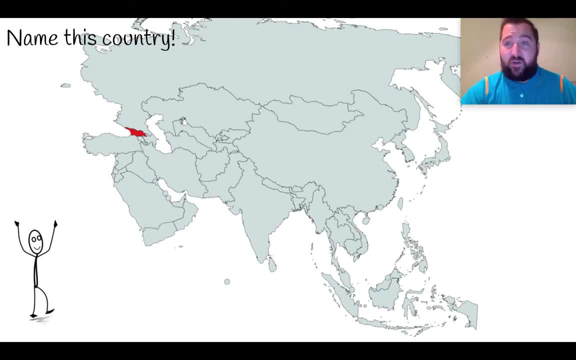 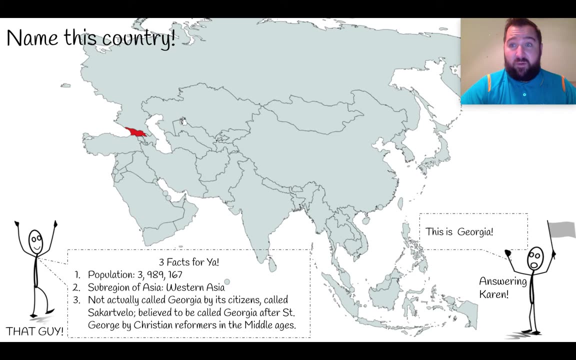 maybe eighth or ninth grade, i had a new student at our school and she told her she was from this country and i felt like an idiot and you'll see why this country is actually called called georgia. and when she told me i'm from georgia i totally thought she was like right above florida. i was. 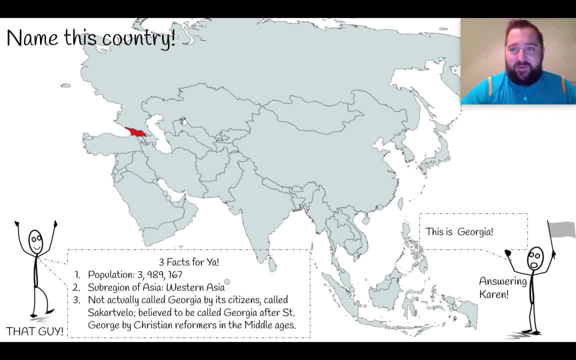 like that's awesome. i'm from florida. uh, i realized- oh, you were. there was a country in the world named georgia. so if you didn't know that there is a country in the world named georgia, here's an interesting fact i want to share with you guys, the people who live in georgia. they don't actually 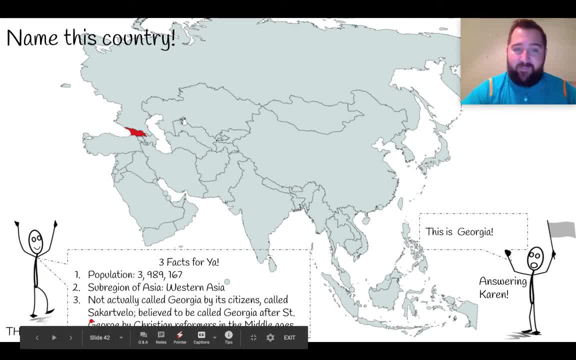 call their country georgia. they actually call it by a different name. i put it down here: called sarca tell velo. um- i don't know if i said that correctly- um, but they, that's not what they call it. we call it georgia, what we believe. you know, historians believe that in the middle ages there 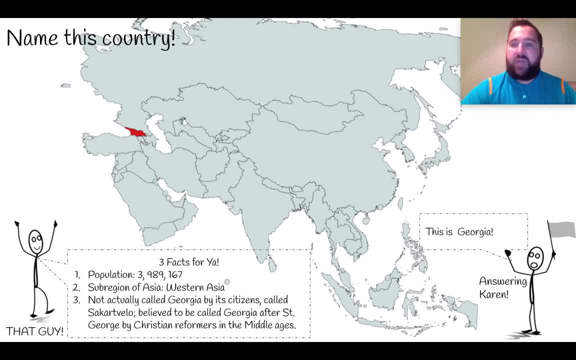 was a, a saint george, and christian reformers name that country after saint george, but they don't call it georgia in their country, even though when she translated to me she told me it was georgia, but she would say to other people: um sarca. 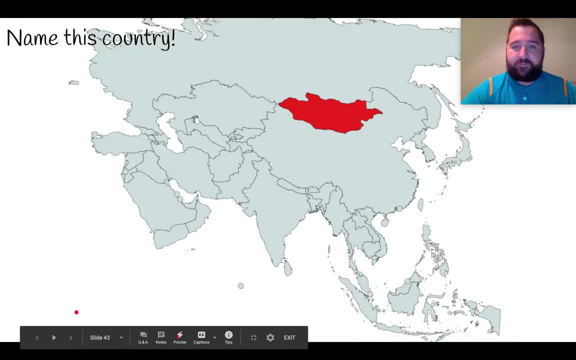 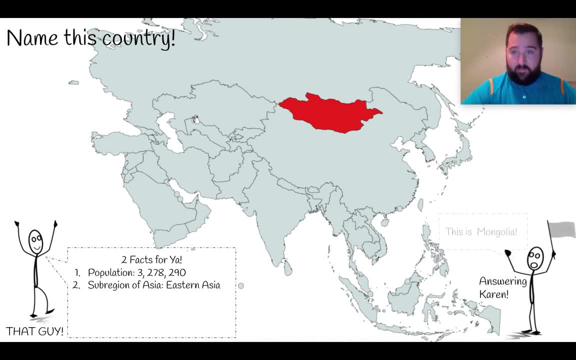 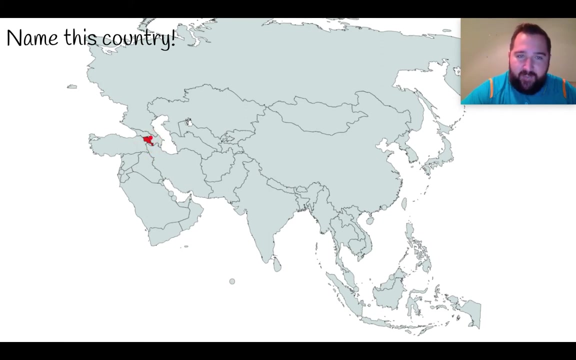 tell velo, but that's pretty interesting. next country up here, big guy on the top. does anybody know what that one is? answer: mongolia. mongolia. population of over 3 million 278 000 290 people. this is mongolia. let's keep going. little little little guy up here. i don't know if you can see that this next country. 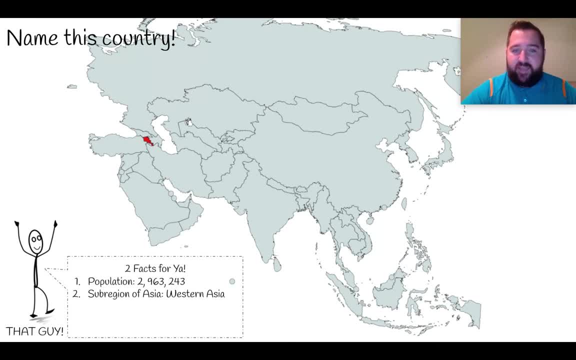 does anybody know what that next country is? this next country is armenia, armenia. many of you have heard of the palestinian, armenian conflicts. um, here we have a population close to 3 million, 2.9 million people. again, this is in western asia. let's keep going. 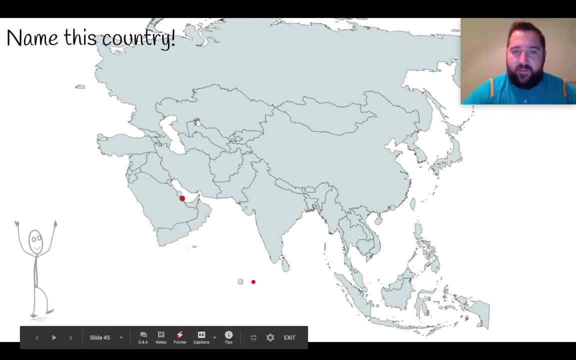 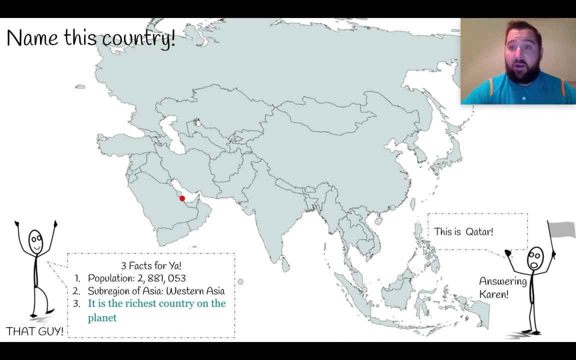 little little guy right here right on the water. does anybody know what that is? that is ready. pronounce qatar, qatar, um. i saw online some people pronounce it. cutter like c-u-t-t-e-r. qatar um clothes. really interesting. did you guys know that qatar is the richest country on the 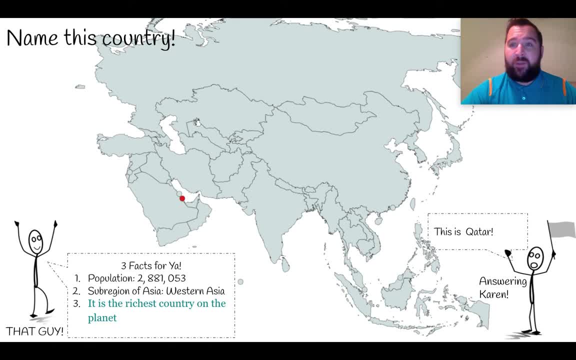 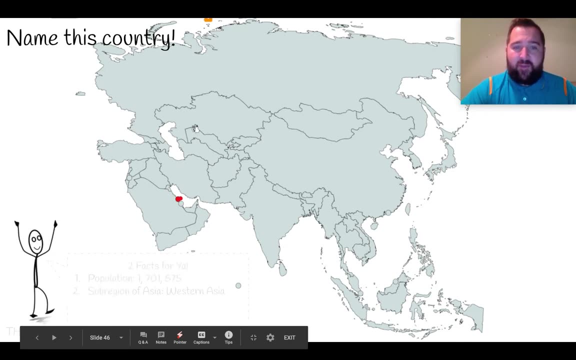 planet. if you have some time, go to google, go to google images and look at some of these buildings and luxury cars and stuff they have over there. a lot of oil, a lot of oil. let me keep going here. next dot here: does anybody know when that one is that one? 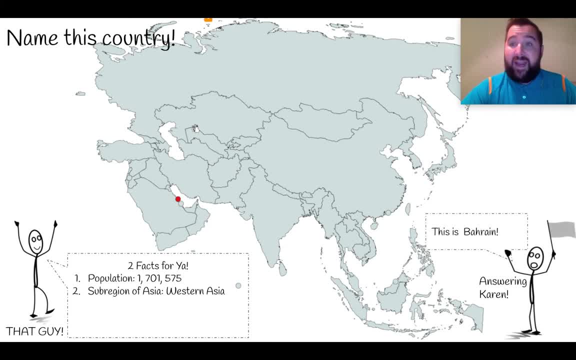 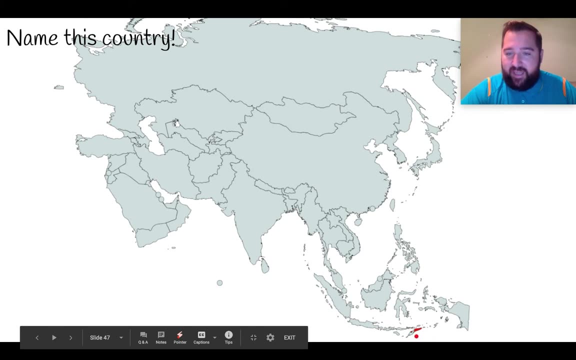 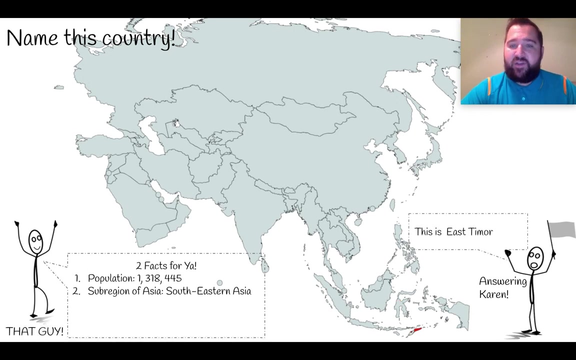 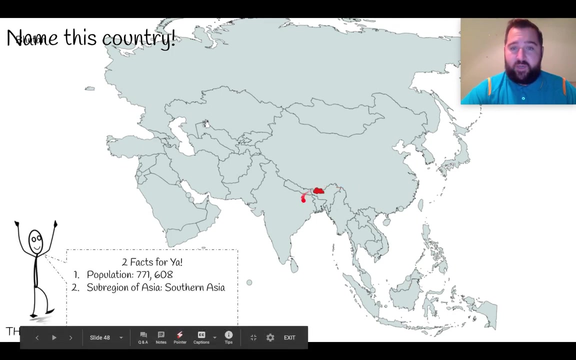 is Bahrain, Bahrain, Bahrain. population: one million seven hundred one thousand five hundred five people. next, one way, way down here, very, very, very bottom. it's actually like, looks like it's a half of a country. this country is known as East Timor, East Timor. this country here is the next one. this country here is known. 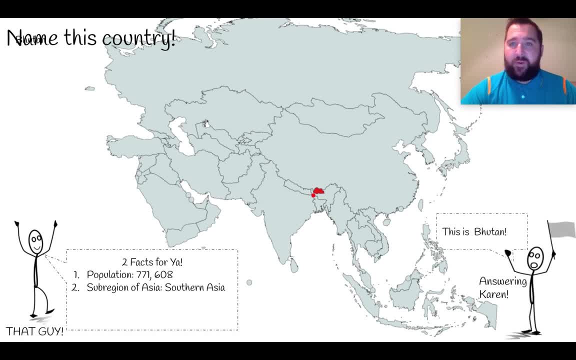 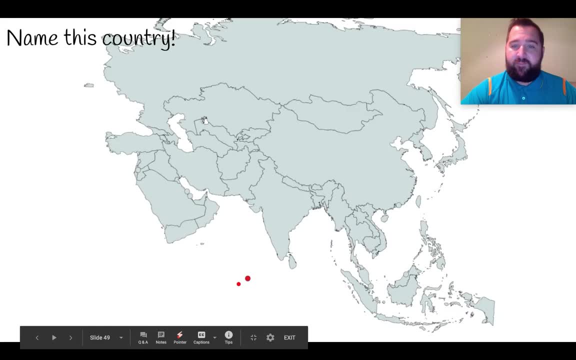 as Bhutan. Bhutan- population less than American million in the sub-region Asia of southern Asia. and our last one, I think the last one or last two right down here. this country is known as Maldives. the Maldives- you may have heard that before- very small population, only like half a.